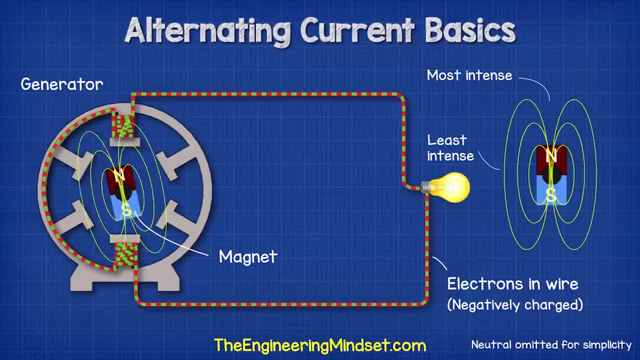 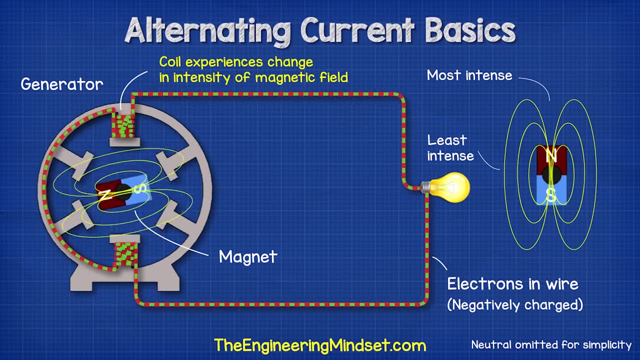 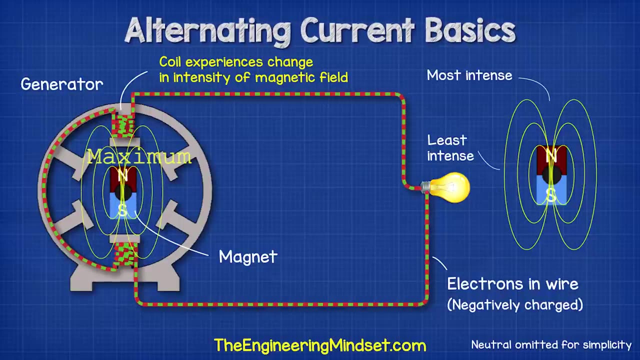 The magnetic field of the magnet varies in intensity. So as the magnet rotates past the coil, the coil will experience a change in intensity of the magnetic field. This will be from zero up to its maximum intensity and then, as it passes the coil, it will decrease again back to zero. 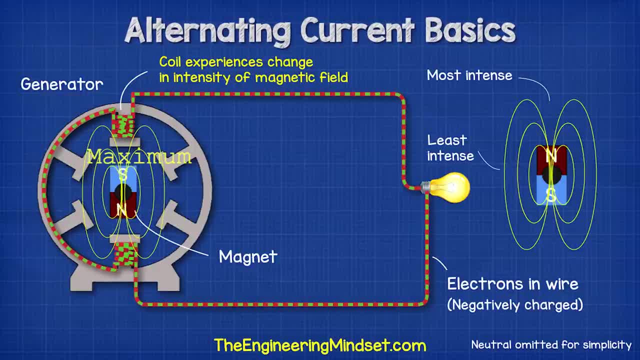 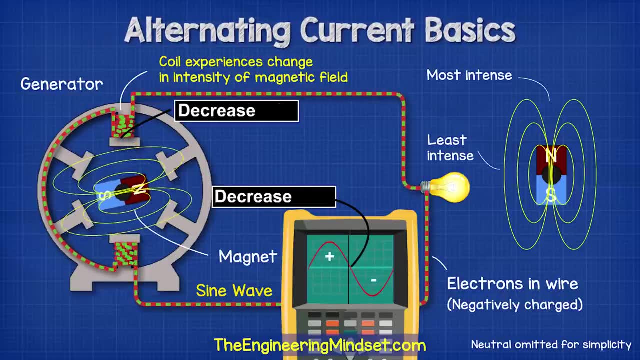 Then the negative half comes in and pulls the electrons backwards with the same change in intensity. Each full rotation of the magnet will change in intensity. Each full rotation of the magnet will therefore produce this wave pattern known as a sine wave. The voltage is not constant in this type of electricity. 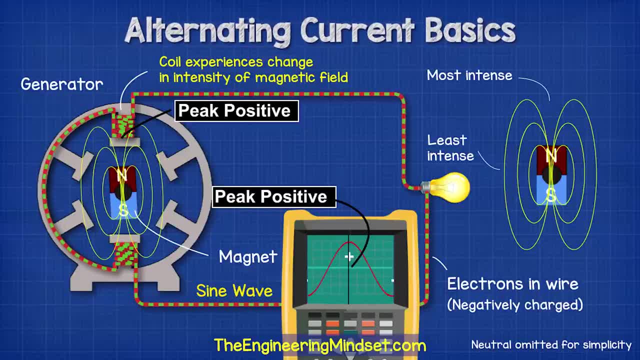 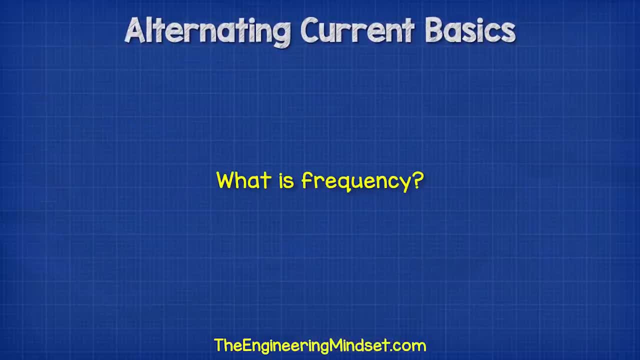 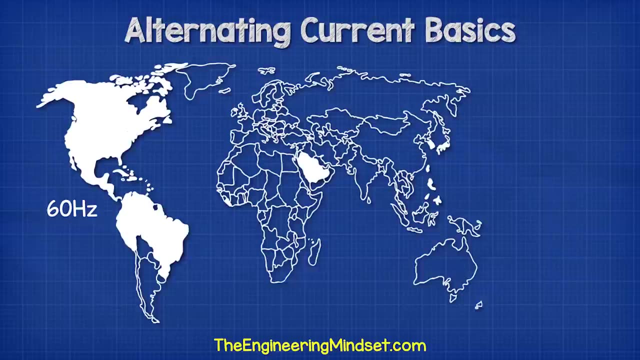 Instead, it repeatedly moves from zero up to its peak, back to zero, then to the negative peak and then finally back to zero again. Frequency refers to how many times this AC sine wave repeats per second In North America and a few other parts of the world. 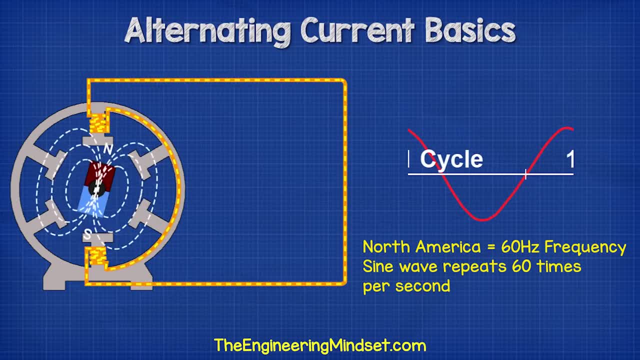 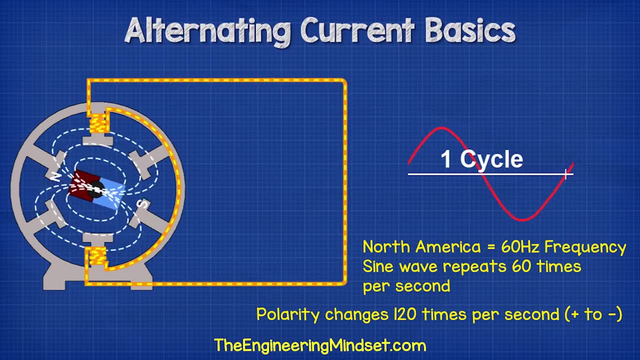 we find 60 hertz of electricity, which means the sine wave repeats per second. The sine wave repeats 60 times per second And as each wave has a positive and a negative half, this means its polarity will therefore reverse 120 times per second. 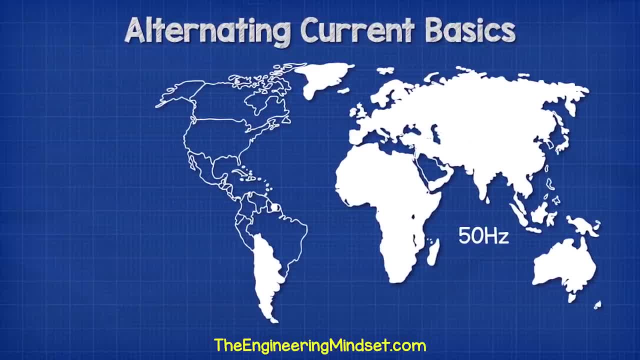 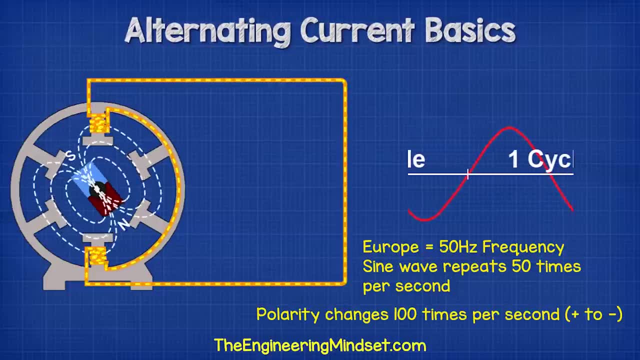 In the rest of the world we mostly find 50 hertz of electricity, So the sine wave repeats 50 times per second and therefore the current reverses 100 times per second. We also have single phase as well as three phase AC electricity. 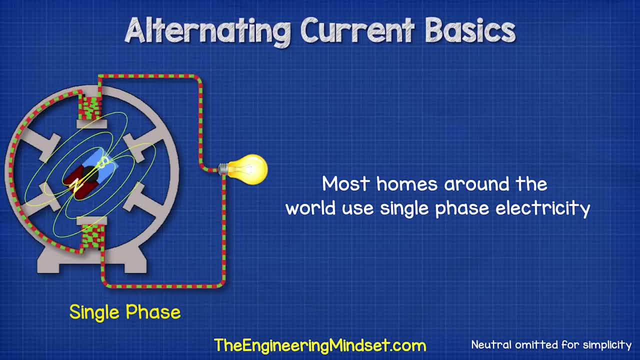 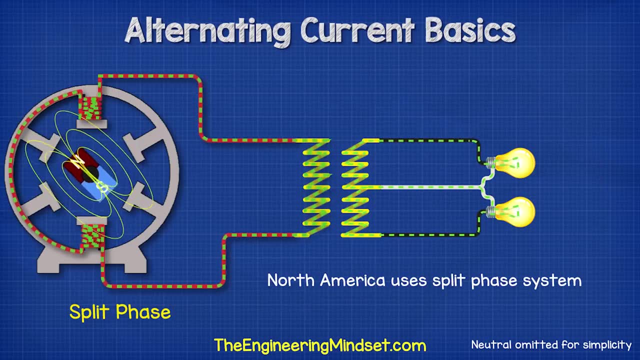 Most homes around the world use single phase electricity. Large commercial buildings, as well as some homes, especially in Europe, will use three phase electricity. Homes in North America use split phase electricity, where a center tap transformer splits a single phase into two. 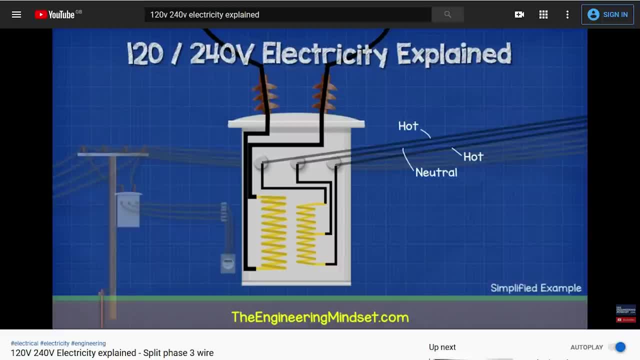 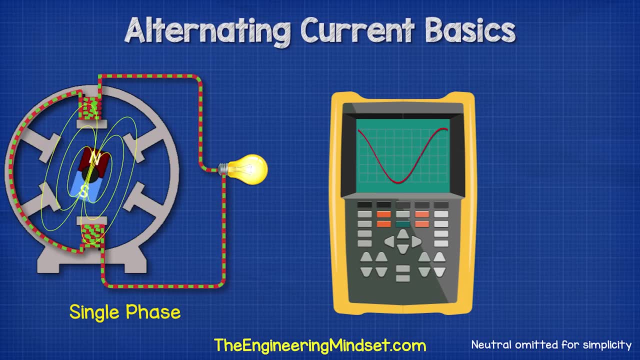 which provides two hot wires and a neutral. We've covered how split phase electricity works in detail in our previous video. Do check that out. Links down below. With single phase we have a connection to just a single phase from a digital power supply. 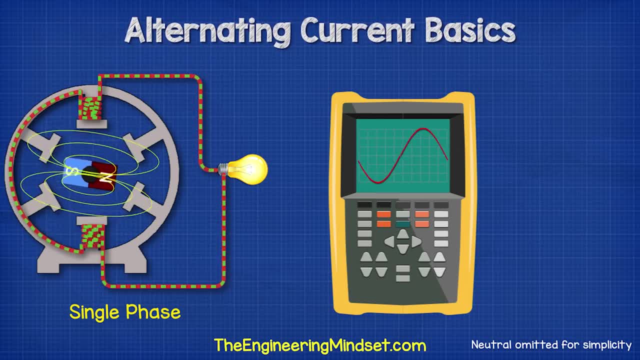 With single phase, we have a connection to just a single phase from a digital power supply. With single phase, we have a connection to just a single phase from a digital power supply. So we have just one sine wave, But with three phase electricity.